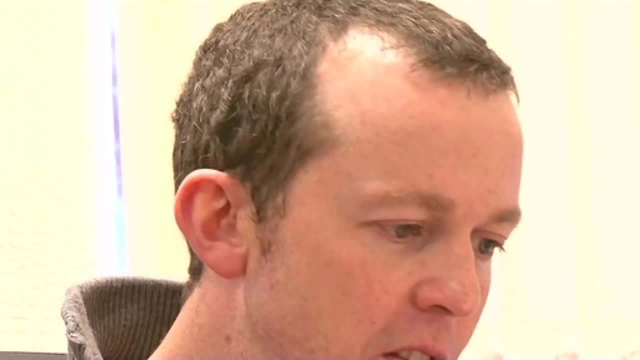 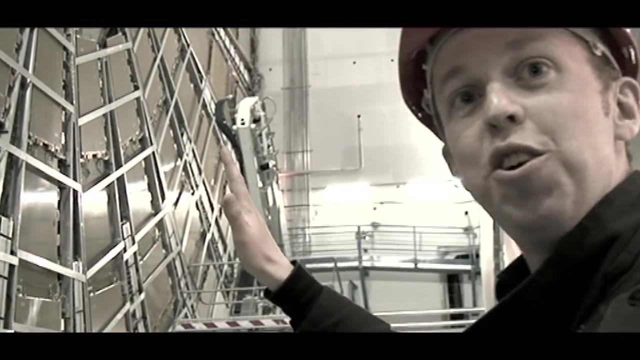 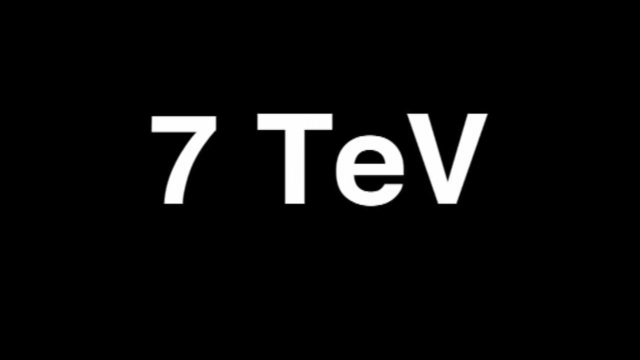 we really didn't know where they came from. Super, super high energy, far, far in excess of any kind of proton that's flying around the LHC, for example. So, for example, at the LHC, protons have around. well, when it's at full whack, which it will be once it starts up again, what we call 7 TeV of. 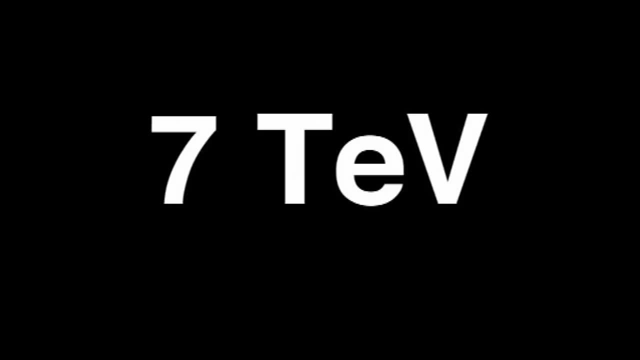 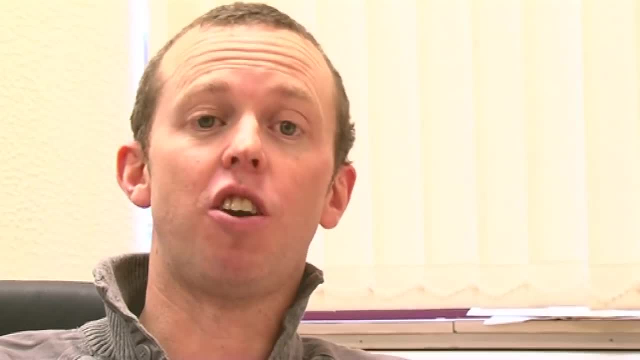 So that's 10 to the 20.. So that's 10 to the 20.. So that's 10 to the 20.. So that's 12 electron volts And basically the ones that the high energy cosmic rays that were coming from outer space. 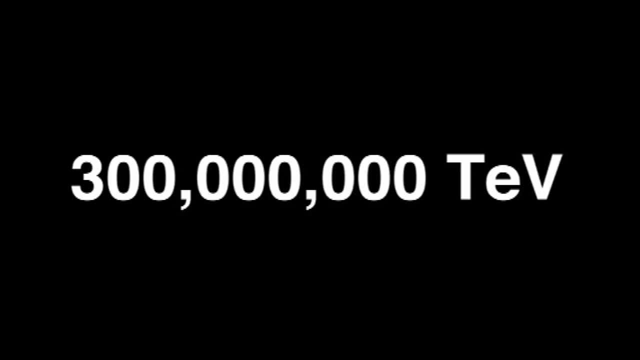 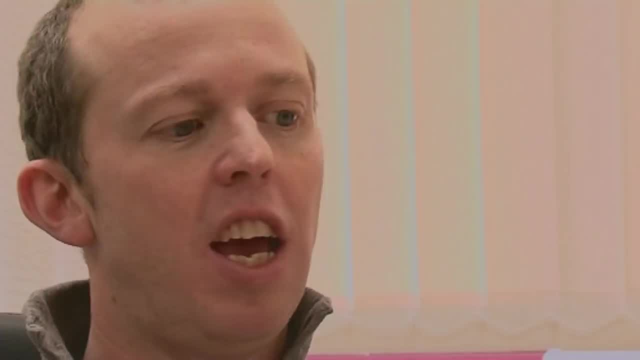 the highest ones have been about 300 million TeV, So an awful lot more. To get a picture of how much energy is installed in those highest energy cosmic rays if I were to like whack a tennis ball at you, Brady, at 100 miles an hour. 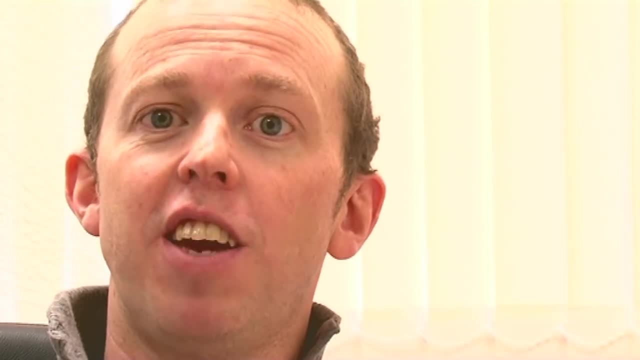 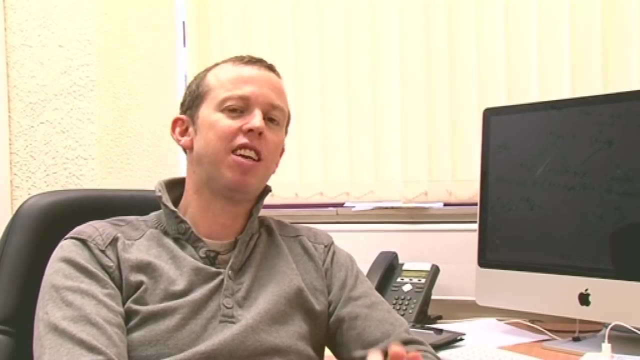 the kind of speeds that you know the top players like Andy Murray's of this world are serving at. that's the kind of energy we're talking about, But it's packed into a single proton, But actually, when it comes to smacking the earth, most of them would just pass straight. 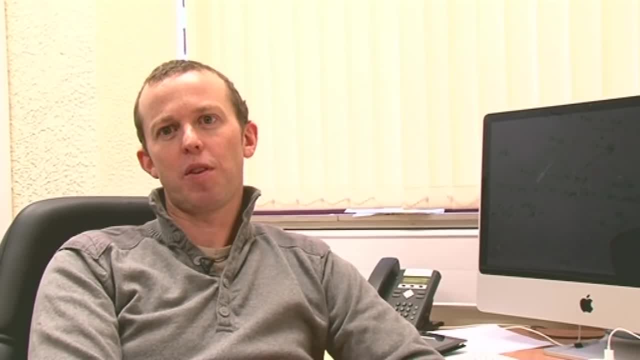 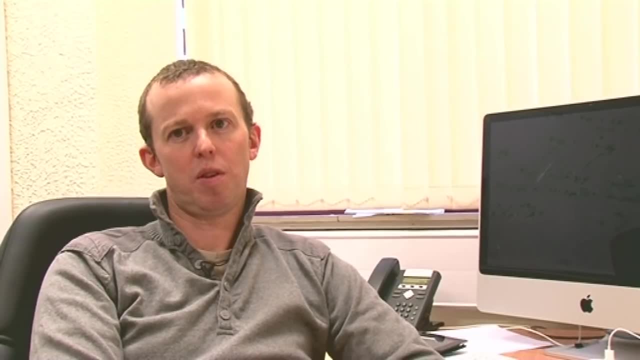 through, because the earth isn't dense enough In most cosmic rays. come through the atmosphere, come past us, go through the earth, go through the core of the earth, come out the other side and keep going through space. Yeah, most of them will pass straight through. 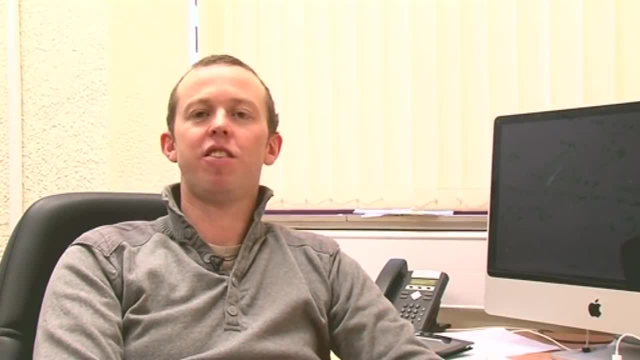 that's correct. Yeah, yeah, It's amazing. Yeah, One of the questions is: so: why do we not know where these things are coming from? We know they're supposed to be very sophisticated. We've known about these things for 100 years Now. 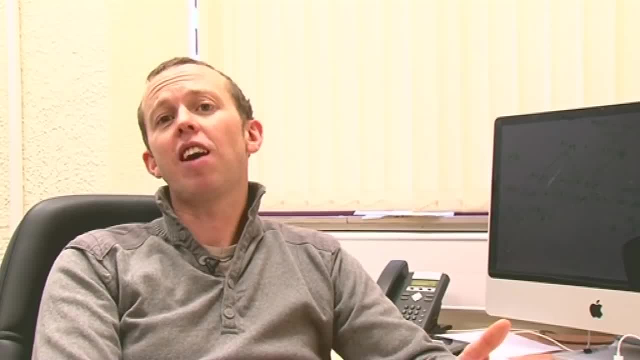 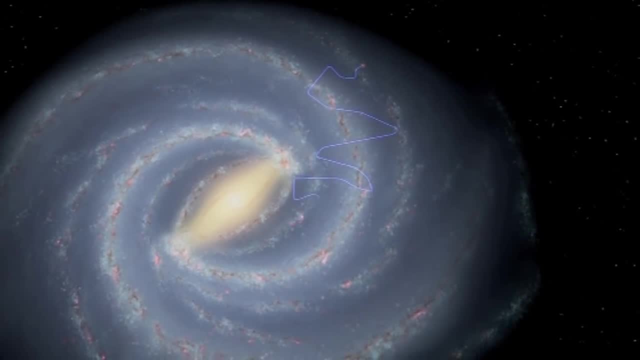 why did we not know where they come from? The problem is these guys are charged. okay, They're protons, they're charged, So charged particles get moved around in magnetic fields and there's a lot of magnetic fields out there in the galaxy and beyond. 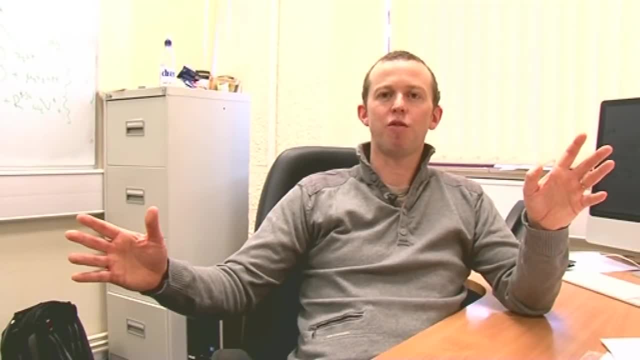 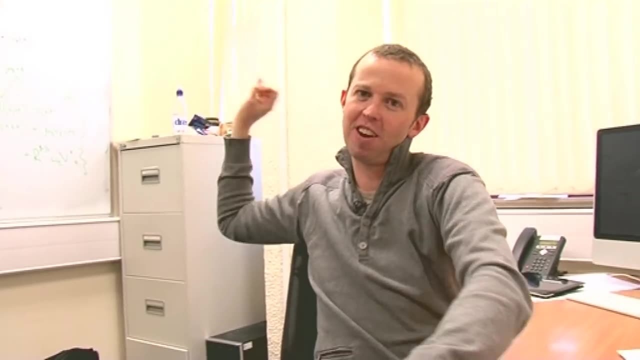 So let's say right, I have some crazy magnetic field going on in this room and there's a proton sitting outside the room and it- you know it- comes through the door, it gets moved around, the magnetic field twists it all the way around. 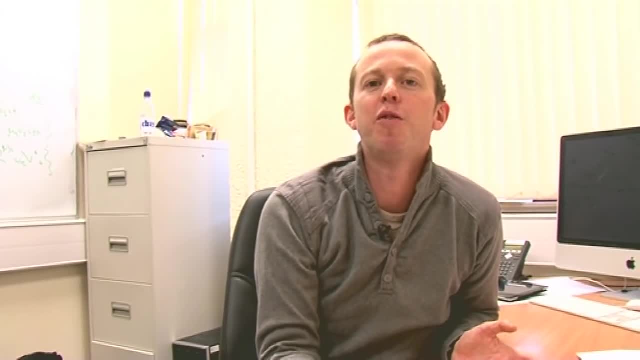 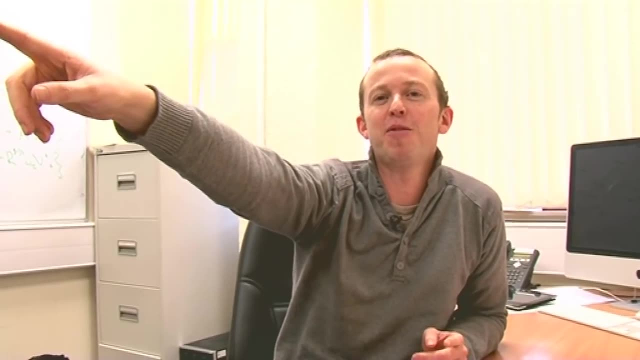 and it goes smack straight into your face, Brady. Which direction did it come from? Well, I'm going to think it came from that way, Absolutely. you think it came from that way, but it didn't. It was hiding outside the room before you even started this video. 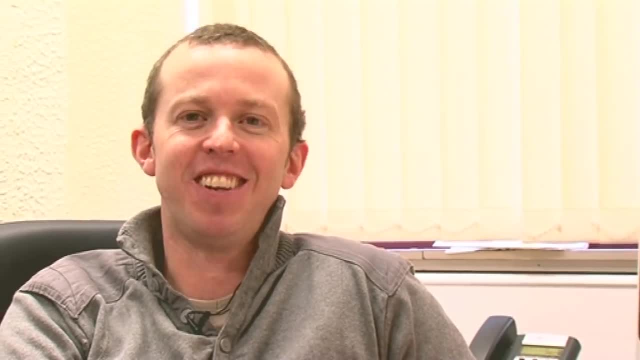 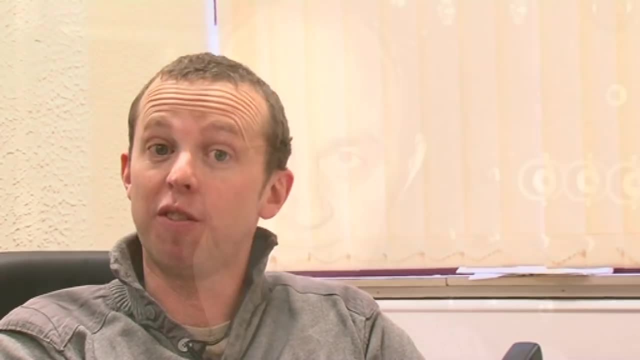 So we throw up our hands in the air and say we're never going to know? No, of course we don't do that. We find other ways to work out where it came from. There was an idea that really dates back to a guy called Fermi And, interestingly enough, 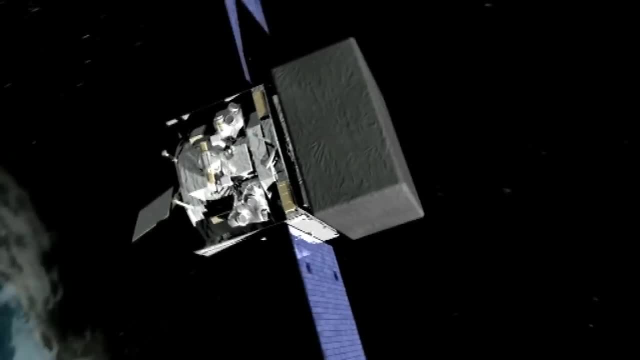 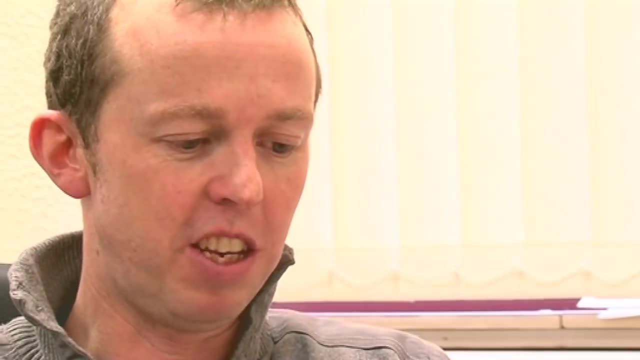 the satellite which has made the observations which led to the discovery that was announced today is also called the Fermi satellite, So it's a nice coincidence, But anyway, these ideas go back to Fermi. What he suggested was that when a star dies, 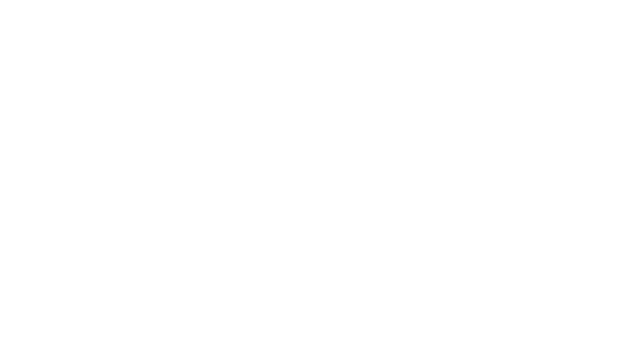 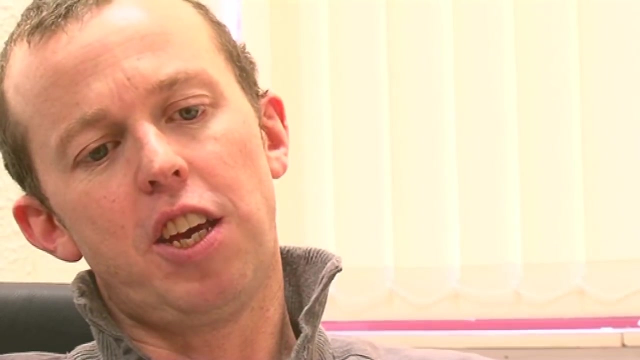 in a supernova. when a star reaches the end of its life, it runs out of fuel. in certain situations it can go supernova, And one of the things that happens with a supernova is that you send out a shockwave- Okay, this very, very powerful shockwave. It basically happens. 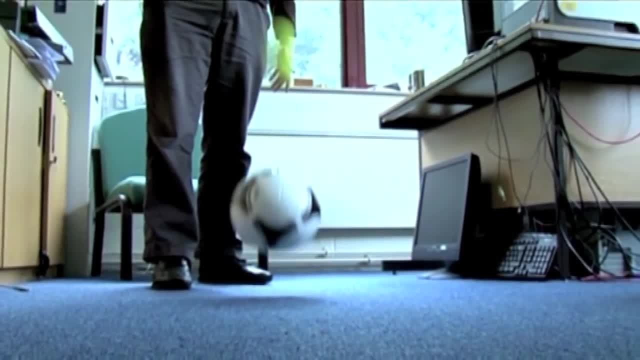 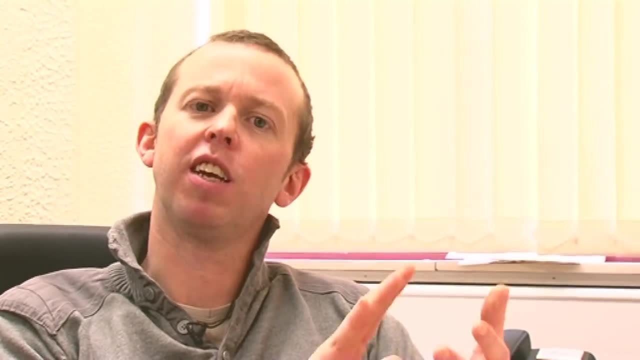 because the star tries to collapse and then it gets. the collapse is sort of jolted by the neutrons in the star not wanting to be put too close together. You get this sharp sort of abrupt halt in the collapse and that causes the shockwave. We will hit the ceiling in a second. 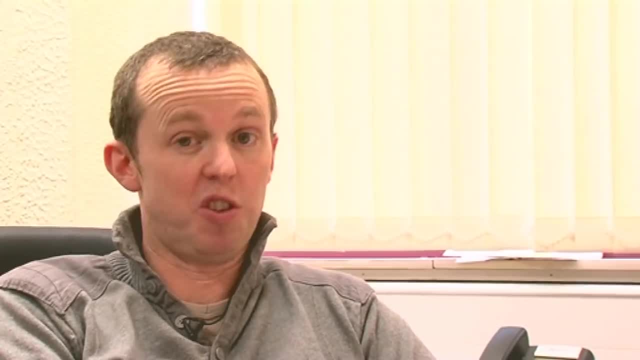 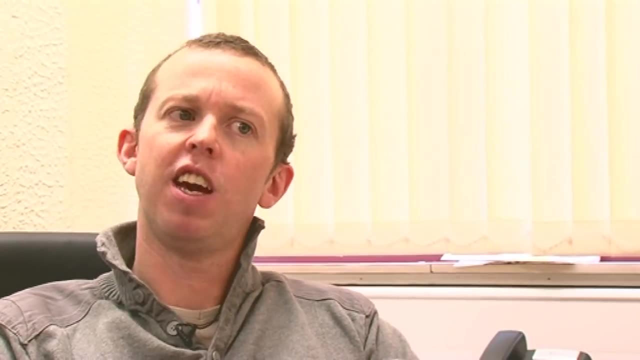 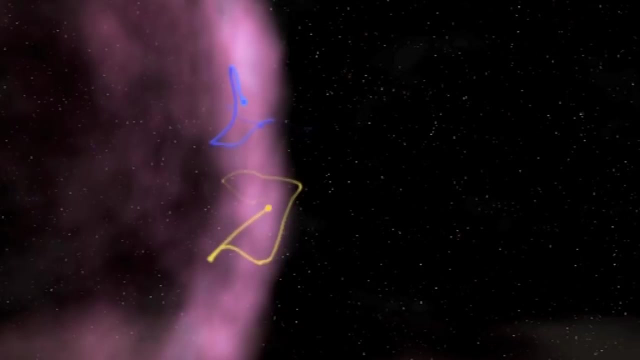 That's what a supernova is essentially, Anyway, so you have this shockwave. you have a situation when you have a proton which is moving around in the magnetic field surrounding this dying star. Okay, so it's moving around the magnetic field. every so often it passes the shock front. 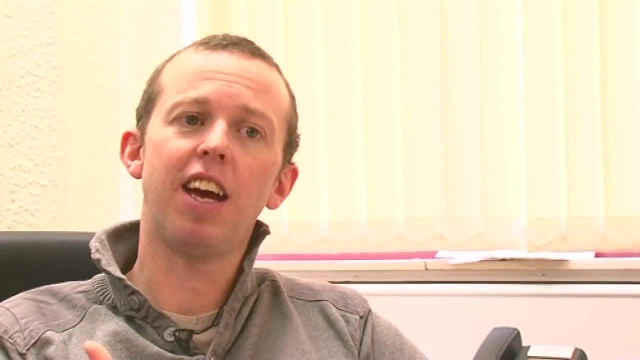 When it passes that shock front, it gets a kick from the shock. Okay, it gets a kick from the shock and it gets accelerated a bit and then it moves around a bit more, going in all higgledey because of this magnetic field. 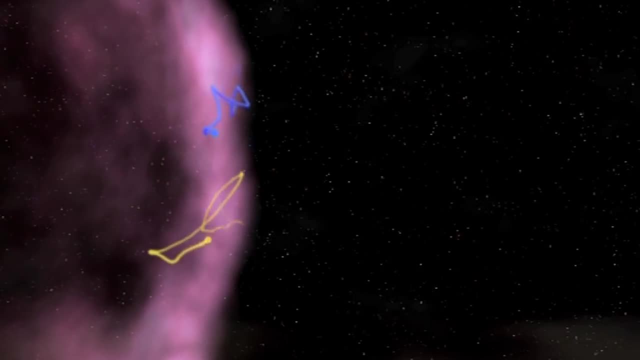 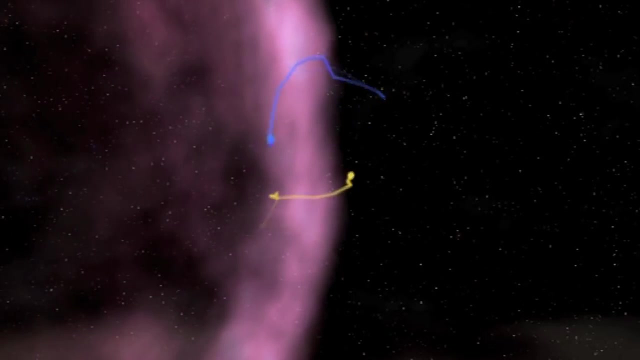 Eventually it passes the shock front again And it gets more of a kick. more kinetic energy. Each time it picks about 1% of its kinetic energy, It increases it by about 1%. So it's getting more and more and more and more energetic. 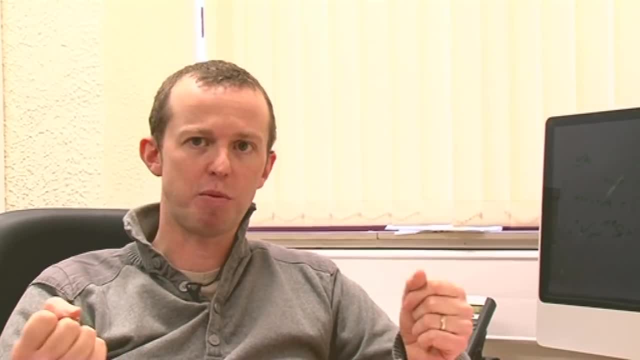 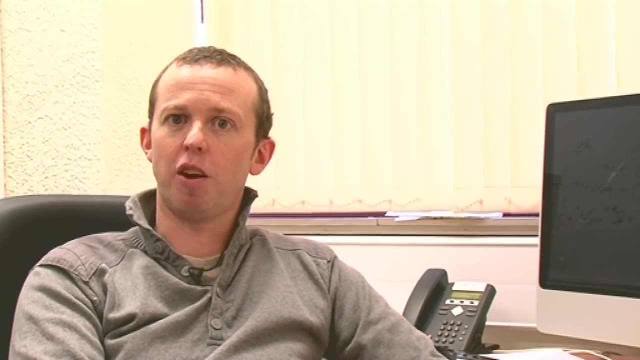 Eventually it gets so energetic that it escapes. This is the idea. This might be the source of high-energy cosmic rays. So we start looking at objects like that. What might we see? So let's look at a supernova and ask: what might we see? 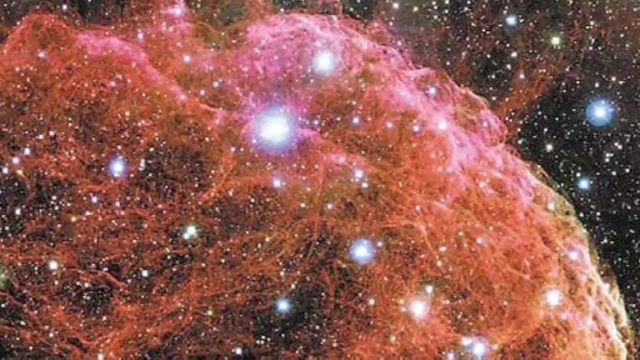 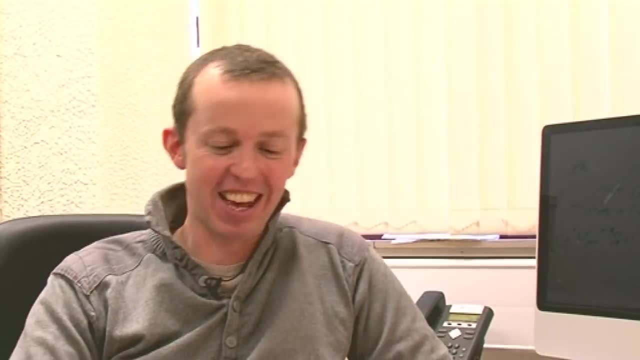 And in particular they looked at two particular supernovae. They got typical astronomers' names which I'm not going to go into. One of them is called the jellyfish nebulae. So that's quite a. at least you can remember that. 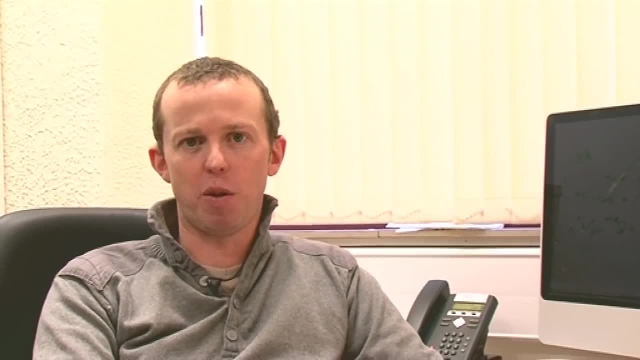 They're both at the order of 5,000, 9,000 light years away, so they're far away objects. These guys have gone to supernovae, so this should be, if this effect is correct, high-energy cosmic rays coming. 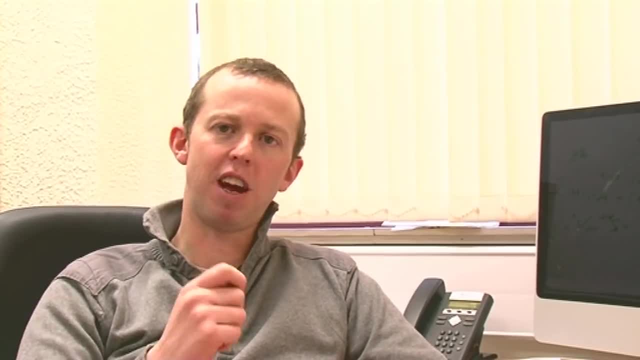 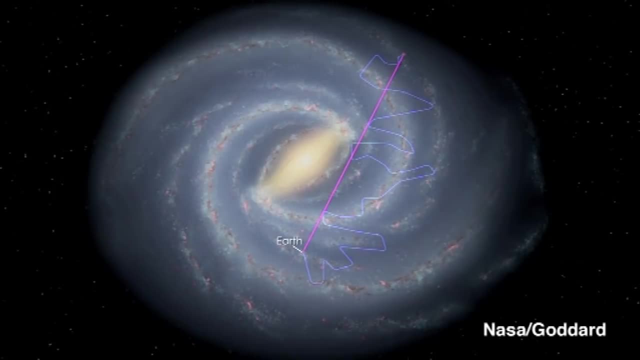 from there. But we're not going to see the protons coming from there because they've moved around so much. But what we can see are photons, because photons don't move around in a magnetic field, Unlike cosmic rays. gamma rays travel to us. straight from their sources. In particular, if you've got a proton, one of these really high-energy protons, what it'll do is, if there's interstellar sort of dust around- there's some interstellar gas cloud or something around this- remnants of this supernova. when the 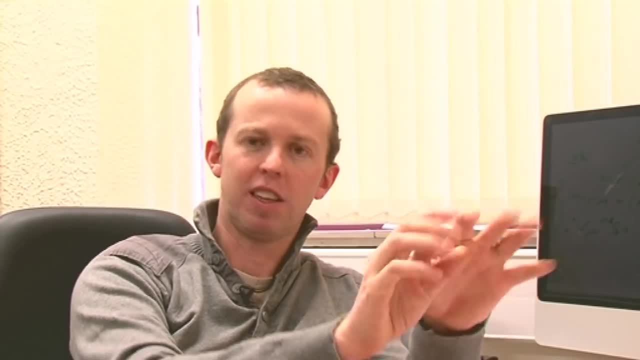 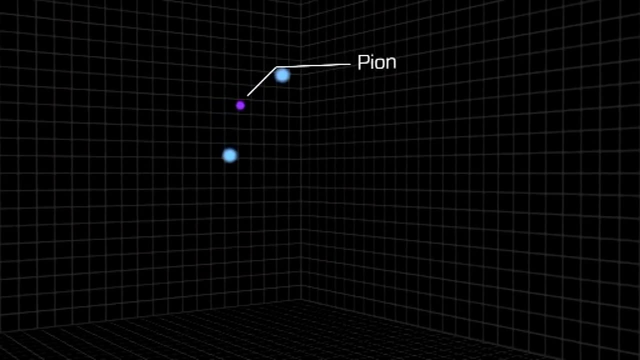 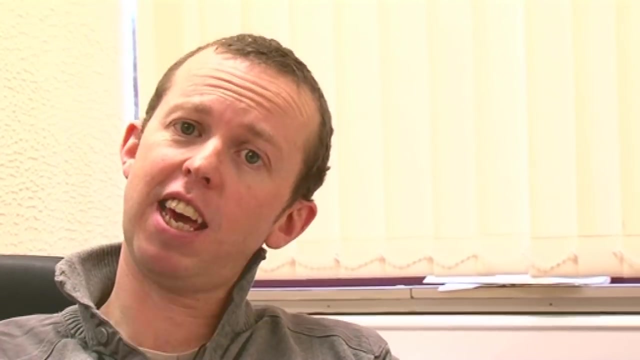 high-energy proton hits another proton that's of lower energy but sitting in this cloud, then basically what'll happen is it can produce what's called a pion. It's a neutral pion, It's just a combination of quarks- So it can produce this pion and then that pion can decay. 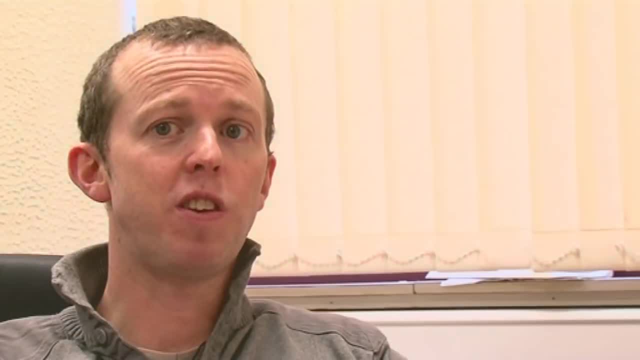 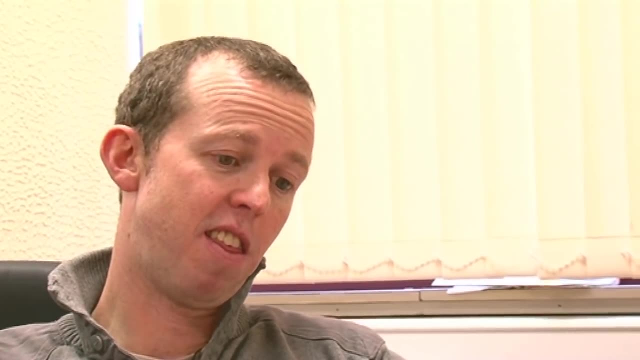 into two photons, and they'll be high-energy photons, And those are the things that we see and those are the things that would come direct to us from this supernova. Now, the important point is that these photons that come from this process have a minimum energy. And the reason they have a minimum energy is because they were produced by the pion itself. So they're at least picking up the energy which is essentially the rest mass of the pion, Which is about 135 GeV gigaelectron volts. 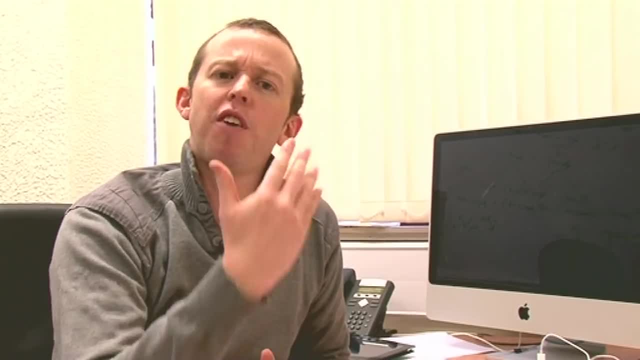 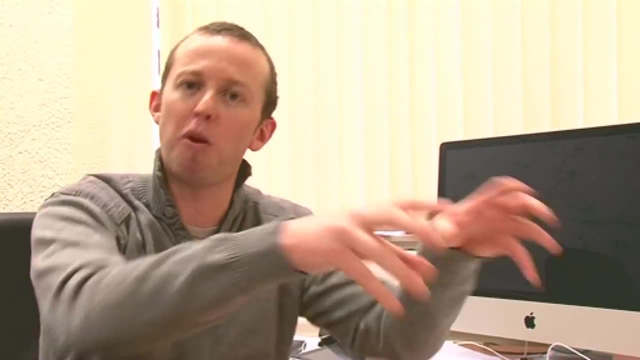 If this effect is correct, you would expect to see a sort of drop in the number of photons around 150, 130 GeV, Because basically, you're not producing them from these pion decays anymore, And so that's what they look for and that's what they saw. 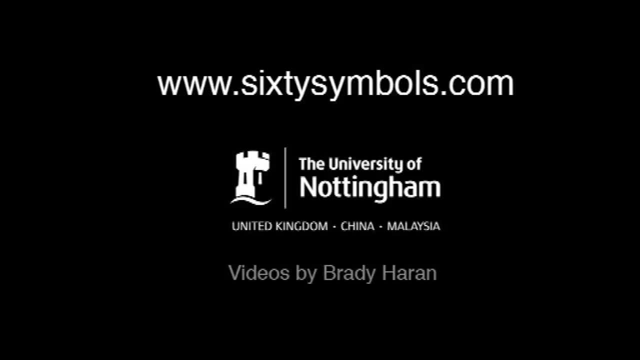 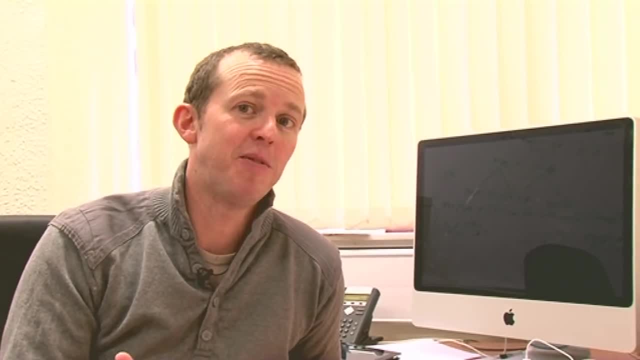 So not the end of the story, Brady, It's so we say we may, so maybe OK, we think this is where it looks like this is where these high-energy guys are coming from. But there is another mystery, And that's that there's something. 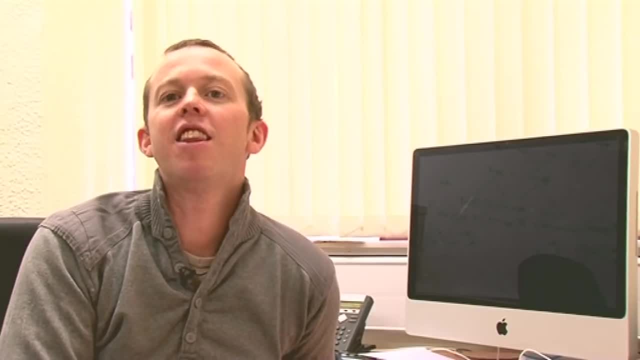 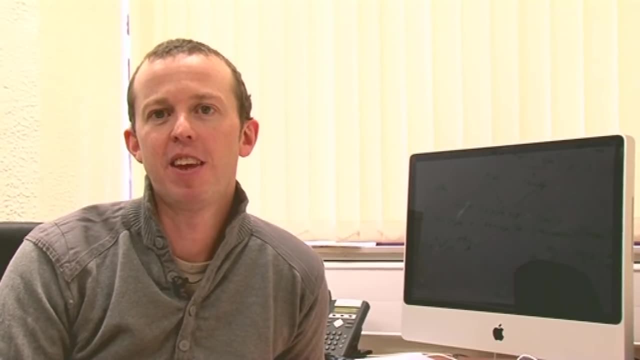 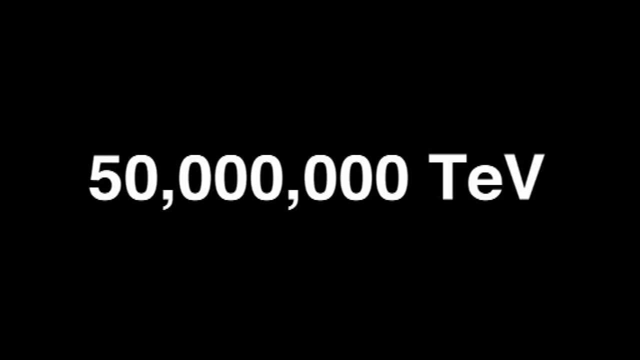 called the GZK cutoff And this basically says that there should be a maximum energy that any high-energy cosmic ray could have. Now it's about 50 million TV Now. remember I said there were ones about 300 million TV, so it's not hugely more. 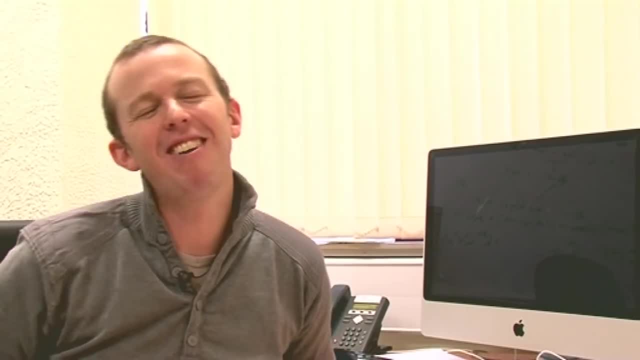 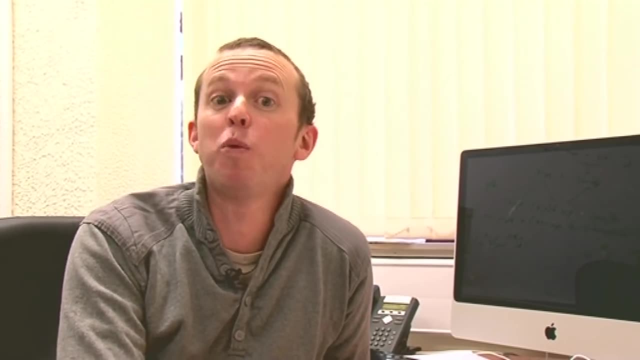 So one could say it's a bit blurry, But it's like six times more. Well, yeah, but six times in cosmological terms isn't so bad, is it? So it's a little bit more, But OK. so why is there a maximum amount that we expect?